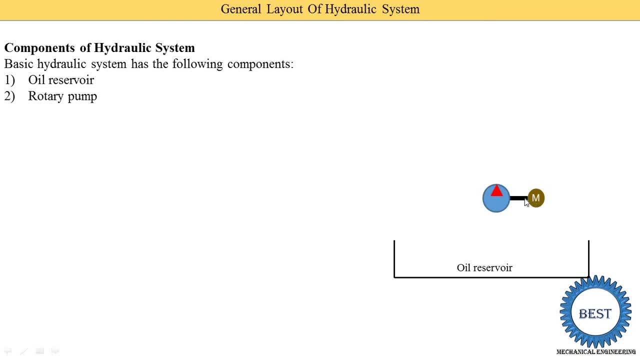 is the shaft. So this shaft is transmitting the power from motor to pump. The pump takes the oil from the oil reservoirs, increases its pressures and then it is supplied to the direction controls. Third component is the pressure relief valve. So pressure relief valve is generally installed. 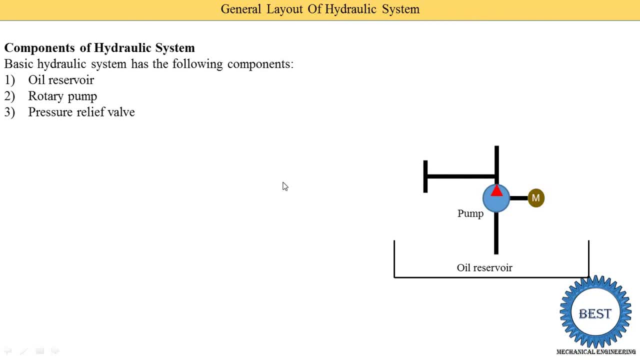 at the outlet of the pump, because it is generally used for the control, the pressure. So it is installed here. that is called as the pressure relief valve. Fourth, one is the direction control valve. So we understand these all the components in the detail later on. First, 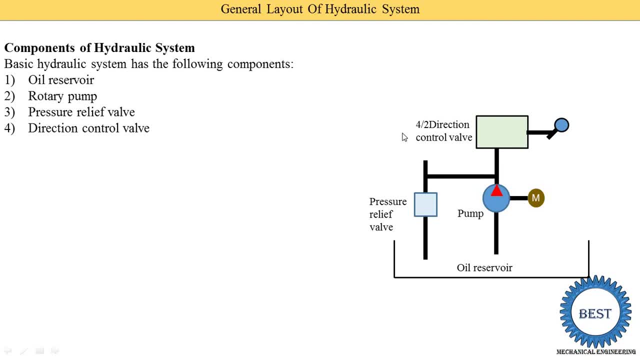 we see the, what are the values? So we make the list. So here you see it is a four by two direction control valves. So it is a four by two control valve means that is a two inlet and two out. let is that. 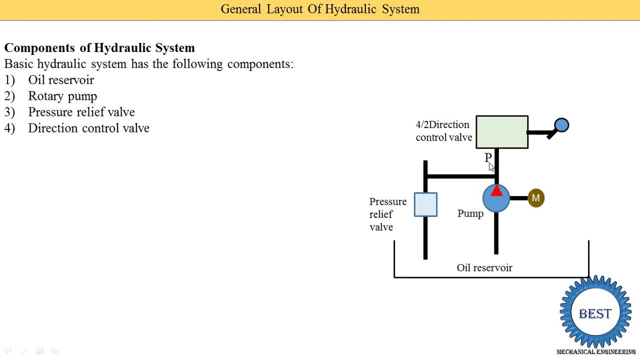 total four value. So this is one inlet that is coming out from the pump, It is the P and it has the two outlets. Okay, it is either supplied to this A or either supplied to the B pipe. That's why it's named- is the four by two direction control valve. Then up the 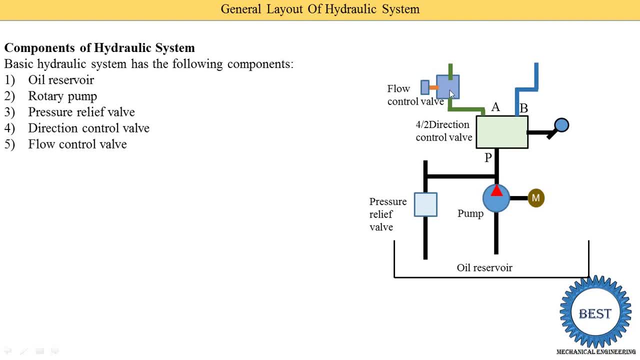 is the flow control valve, so flow control valve is provided here. okay, so here you see, it is the flow control valve. then next component is the double acting cylinder. here you see, it is the double acting cylinders. why its name is double acting? because inside the cylinder, here you see. 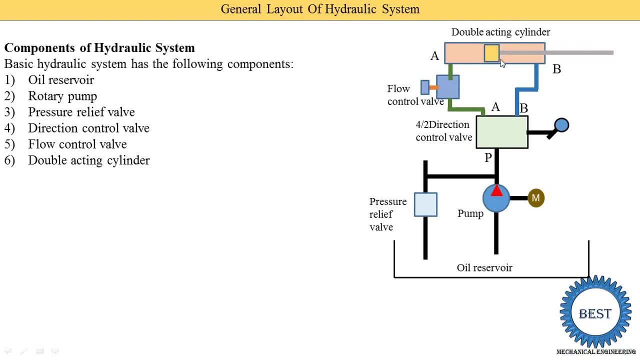 this yellow color component is the piston and the oil is supplying both the side of the piston. that's why it is called as the double acting cylinders. so oil is either supply a sides and a b side- okay- or it is supplied on both the sides. next component is the pressure gauge. so pressure gauge. 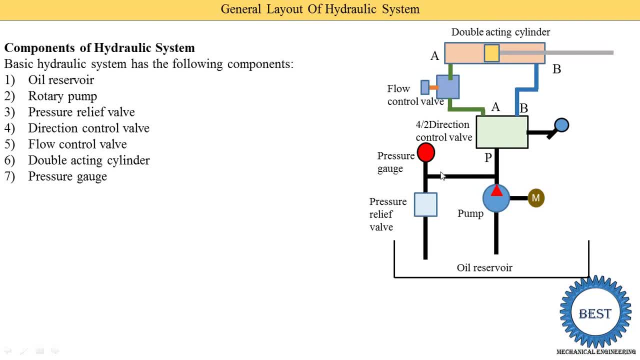 is also installed at the outlet of the pump. so here you see, it is the pressure gauge, and the last component is the filter. so here you see, this is a 4 by 2 control valve. okay, so here the 4 valve is provided and its name is the t. then this oil return is supplied to this filter here. 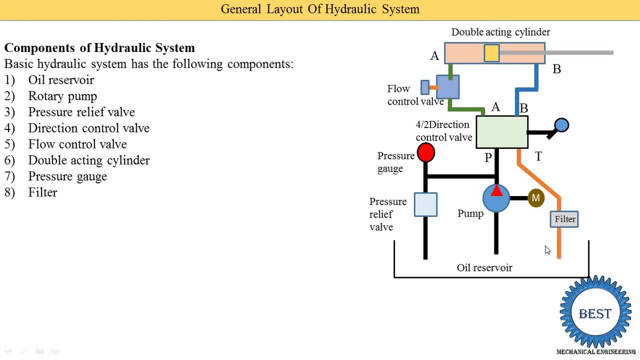 okay, so this component name is the filter. okay, in a sub-component name it is the filter. okay. so here you see it is the filter. okay, so here in the王sw length, here you see the filter. okay, so here the filter. In some book the filter is provided at the inlet of the pump. okay, in a some book it is. 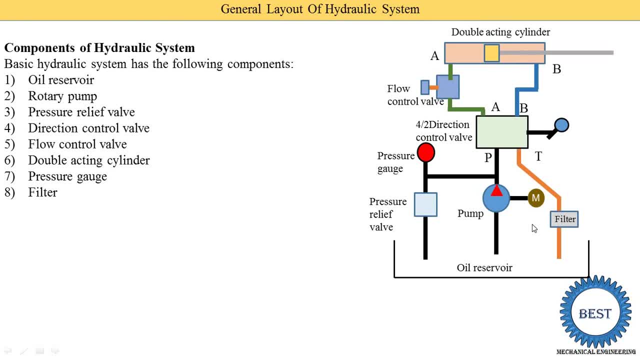 provided at the outlet of the pumps. sorry, not Today, but it is at the return pipes. If you see the filter here at the inlet of the pump, this is also correct. now we understand all the component in the details. first component is the oil reservoir. okay, so here in. 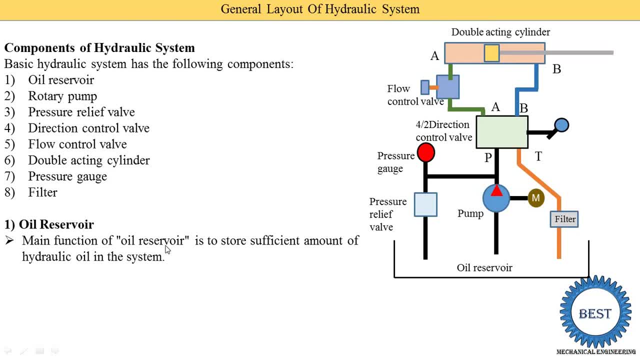 this image you see at the bottom, the oil reservoir is provided. so main functions of the oil is to store sufficient amount of the hydraulic oil in the system means it is generally used for the storage of the oils- okay, in a bike or car. what we are doing? we are the store the petrol. 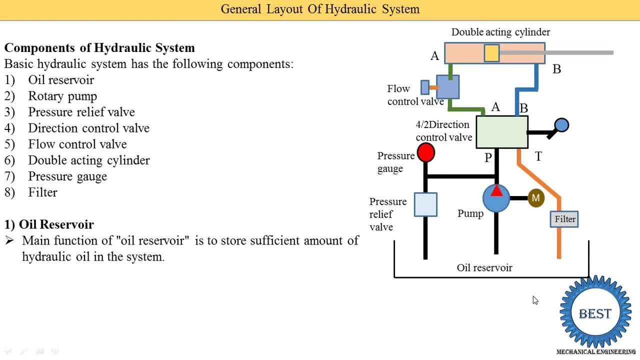 or diesels in the our car tanks. so, similarly, it is the one of the storage place for the oil, because in a hydraulic systems we know that the liquid is used and generally we are use the oil as a liquids, okay- and in pneumatic systems we use the air. apart from this, it has the another 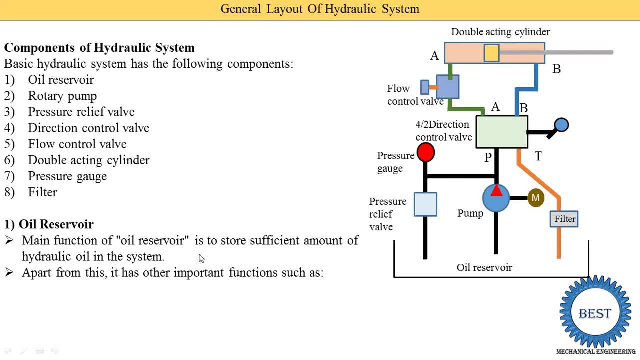 important function such as means. apart from the store of the oil, they have also some another functions. first one is to control the hot return oils. here you see, these are. the return oil is coming, so return oil temperature is increased in this various part or various components, because 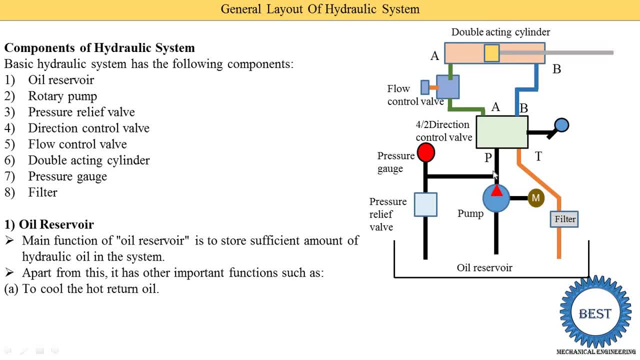 in a pump, its pressure is increased, so with this pressure its temperature is always high. so it is a very important function. so it is a very important function. so it is a also increased. due to the friction in these different pipes and then different component. its temperature is also increased, so return oil temperature is higher, so its temperature. 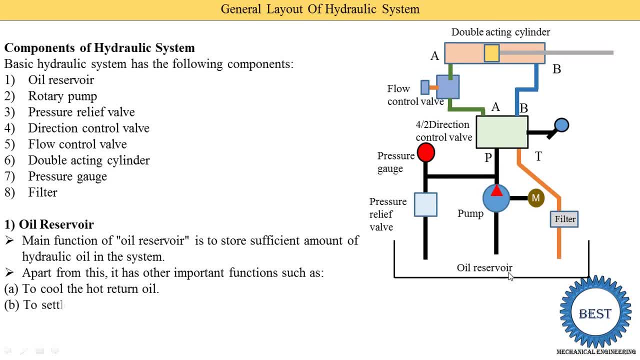 reduction is also required and it is carried out in the oil reservoirs. next function is to settle down the contaminates. so, due to the wear and tear, some of the parts are wear outs. okay, so this metal part is coming out with the oils. okay, so we need to remove this part. it is called as: 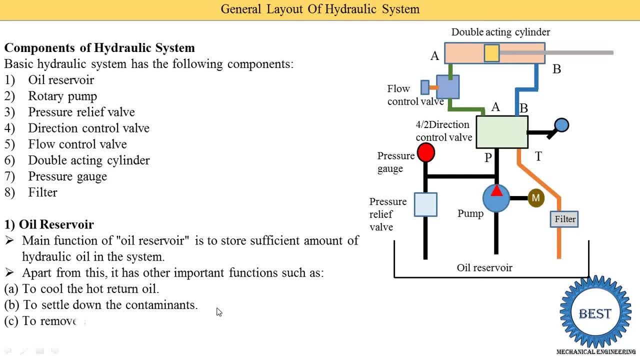 the remove or settle down the contaminates. to remove the air bubbles. why: the air bubble is create in a while, so when the temperature of the oil is increased, so by default there is possibility of the bubble is created inside the oils. so we need to remove this oil bubbles or air bubbles. 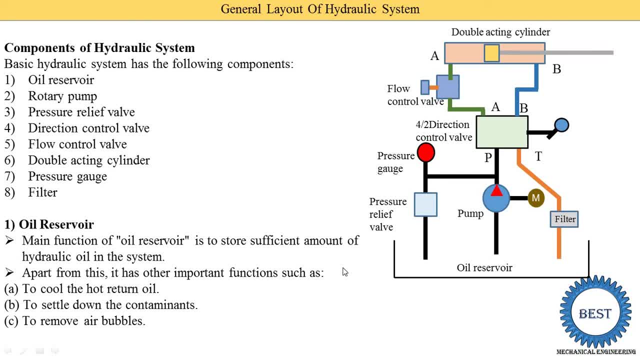 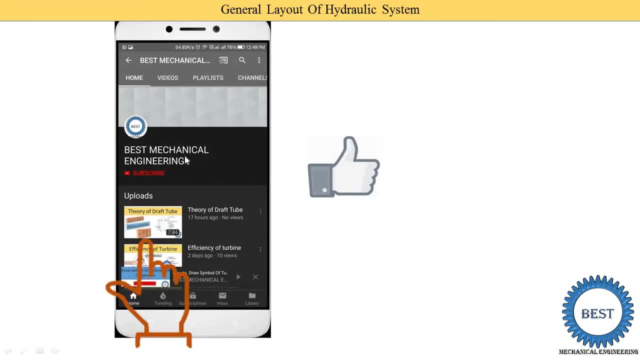 from the system. next point is to separate the water from the oil, so it is oil water also carried out in the oil reservoirs. now, before moving ahead, I request to like the video and subscribe my channels for watching the more video related to oil, hydraulics and pneumatics. 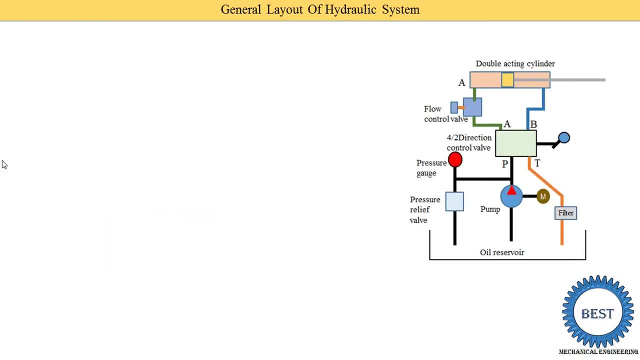 and other subject of the mechanical engineering's. for the more video, I request to visit the playlist. second component is the rotary pump. okay, so why the rotary pump is required? in a oil hydraulic system, we required to increase the pressure pressure. without increasing the pressure, oil are not able to create the much, much force. 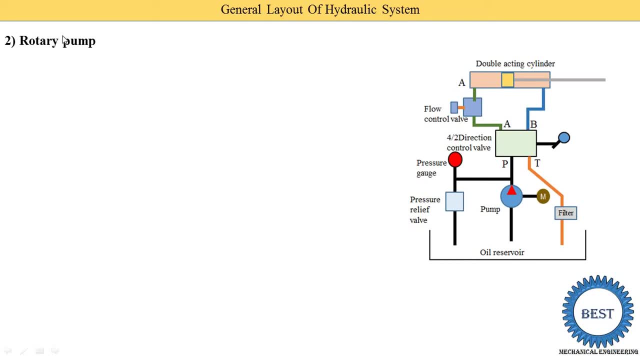 okay, so if you increase the pressure then the force is increased. okay, the functions of the rotary pump is to pump hydraulic oil to the hydraulic circuits means pump its suction, the oil from the oil reservoirs, increase its pressures and this high pressure oil is supplied to this hydraulic circuit. okay, so these all the part is known as the hydraulic circuit means this: 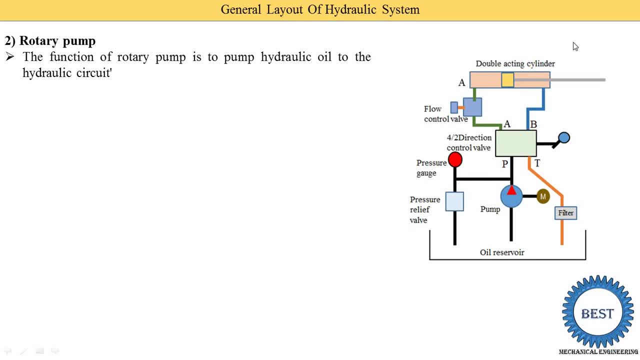 pressurized oil is supplied to direction control valve and flow control valves and double acting cylinders. okay, so this is part. is called as the hydraulic circuit. it converts the mechanical energy into a hydraulic energy. okay, so mechanical energy means it is the rotation of the shaft, okay. 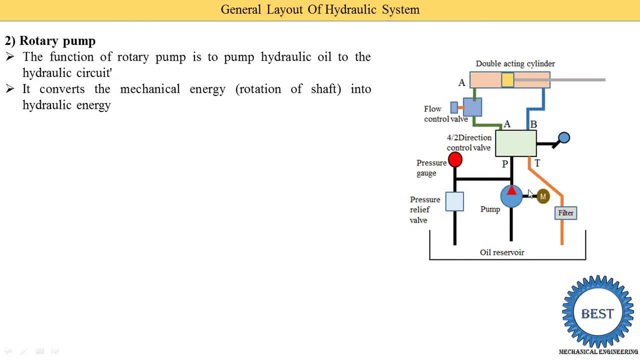 so in a pump- here you see, it is the shaft, okay, and the shaft is rotated. it is called as the mechanical energy. okay, so how we create the mechanical energy. so we have generally available electrical energy. okay, so what we are doing: we supply the electrical energy to the motor, so motor converts electrical. 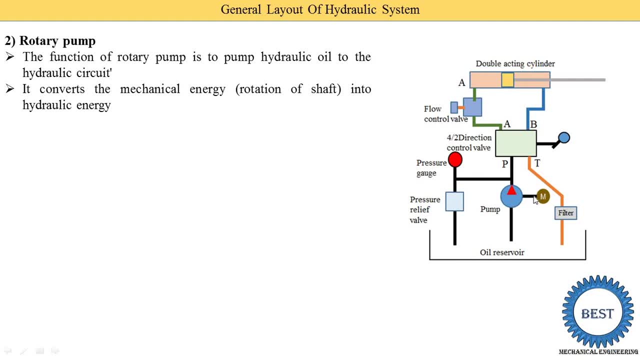 energy into the mechanical energy and this mechanical energy is supplied by the shaft to the pump and pump its convert this mechanical energy into the hydraulic energy. rotary pump is a positive displacement pump. okay, so that is the various type of pump is available. okay, so it is not necessary to use the rotary pump in hydraulic systems. you are able to use a. 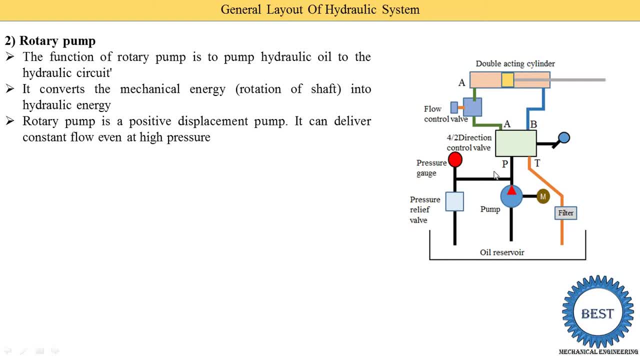 to use also another type of the pump. okay, but in this image we discussing about the rotary pump is the positive displacement pump and it can deliver the constant flow even at the high pressure. so rotary pump is delivered at the oil at the constant flow even at the higher pressures. third component is: 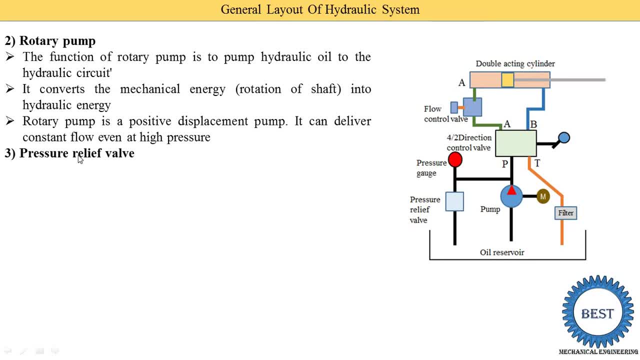 the pressure relief valve. so if you understand this meaning of word, that is a pressure relief valve. the relief means reducing some work. it is called as the relief, now here the with the relief pressure. what is used? so pressure relief valve is used to reduce the pressure of the oil. 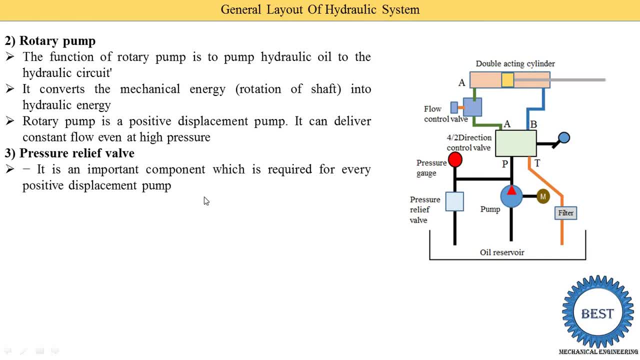 so it is an important component which is required for every positive displacement pump. okay, so here you see that pressure relief valve is attached with this outlet of the pump. okay, this valve is connected at the outlet of the pump and its main function is to release the oil back. 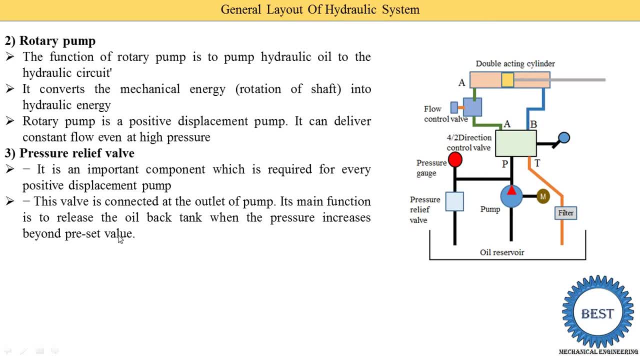 to the tank when the pressure is increased behind the preset value. suppose we are required 10 bar pressures in our hydraulic circuit. okay, but due to some circumstances the pump is delivered the oil at a 12 bar pressure. okay, but what is our desired pressure is the 10 bar, okay, so what? 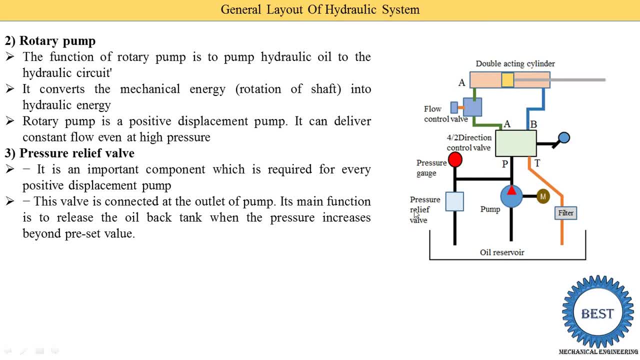 we are doing for this pressure is reduced by using this pressure relief. okay, so first, the pressure is measured by using this pressure gauge. okay, it is the pressure is the about and whatever. okay, so we require 10 and the pressure is the 12 bar. then what happened? the pressure gauge is. 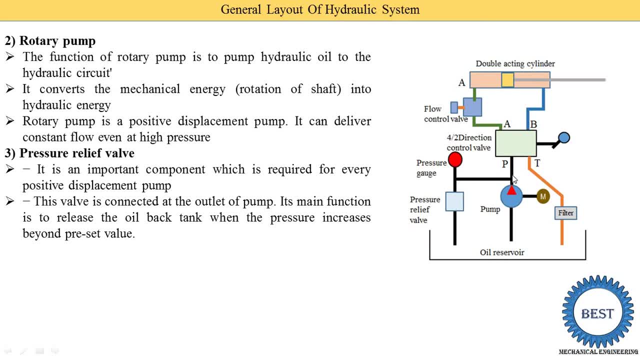 give sense to the pressure relief valve and the pressure relief will take the some quantity of the oil back and supplying to the oil reservoirs. that's where the pressure at the outlet of the pump is reduced to a 12 bar to 10 bar. next is the direction control valve. so from this name, 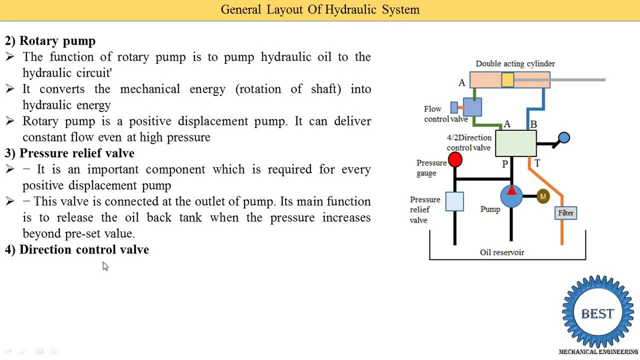 you can also understand what is the meaning of direction control valve. it change the direction of the oil or guide the oil in a proper direction. okay, you are going in these directions, you are going into these directions. okay, so oil is suggest. sorry, the direction controller suggest to oil: to 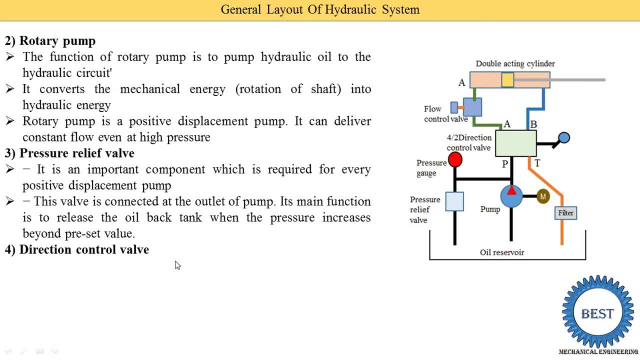 move in these directions. okay, so it is not necessary that the oil coming out from the pump is only supplied to the one single systems. okay, so here you see, we use the double acting cylinder. so we require to supply the oil in two directions: either through the pipe a or either through the 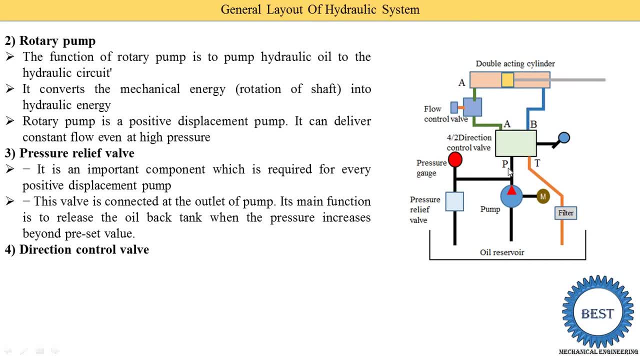 pipe b. okay, so how the oil is going for that we decide by using the direction control valve. okay, so sometime oil is supplied to through pipe a, sometime oil is supplied through pipe b. okay, so it controls the direction of flow of oil, by which it performs extensions and retractions of the 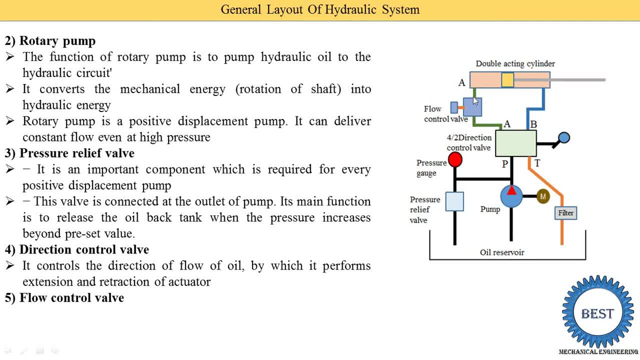 equitators. next component is the flow control valve. okay, here you see, this is the flow control. so from from its name we also understand it's controlled the flow. then if I that's why its name is the flow controller, what is the meaning of flow control? flow means it's controlled the quantity of the 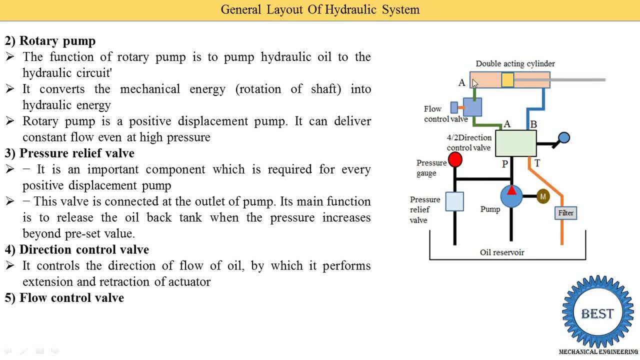 oil supply to this cylinder. okay, this cylinder is one type of the accutator that we understand in the next next points. okay, so sometime the oil supply to the cylinder is required to two meter cube per minute- sometimes the sorry two liter per liter per minute- sometime it's required 2.5. 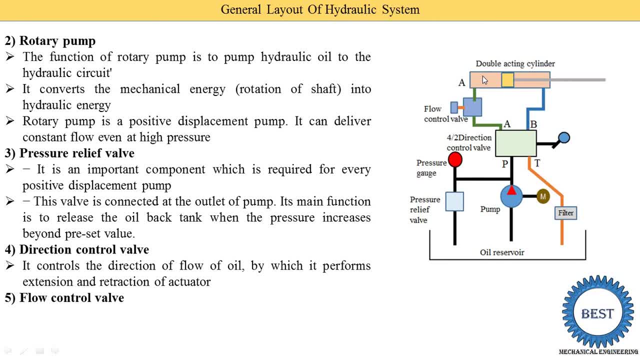 liters. sometime it's required 3, 4 or 5 liters. so it is controlled by using the flow control, while depending on the pressure or a force required. so it controls the rate of flow of oil, by which speed of extensions or retractions of accutator is controlled. this accutator means 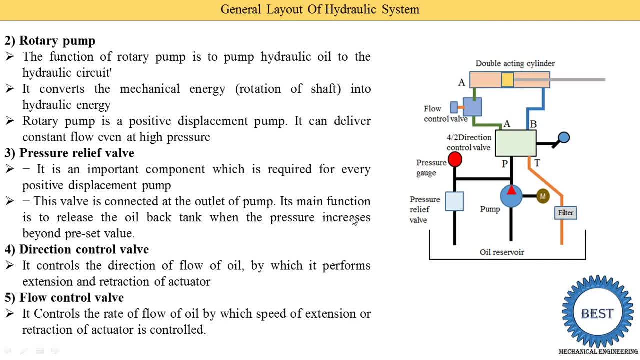 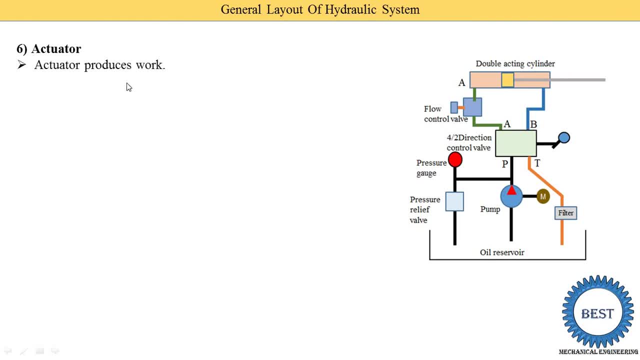 it is a double acting cylinder so you not need to. the confuse. next part is the accutators. accutators produce the work. okay, what is the work? work means it's produce some mechanical work, okay, and what we supply, the supply energy to these accutators? okay, so this double acting? 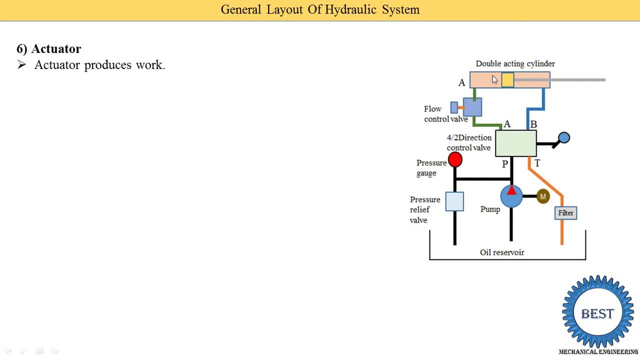 cylinder is over accutators in which we supplied the hydraulic energy. okay, so what happen? in accutators, hydraulic energy is converted into the mechanical energy. okay, and here in the pump, what happen? we supplied the mechanical energy and it is converted in hydraulic energy. okay, so what is the? our system is that we take the oil from here, that is a hydraulic energy, and we 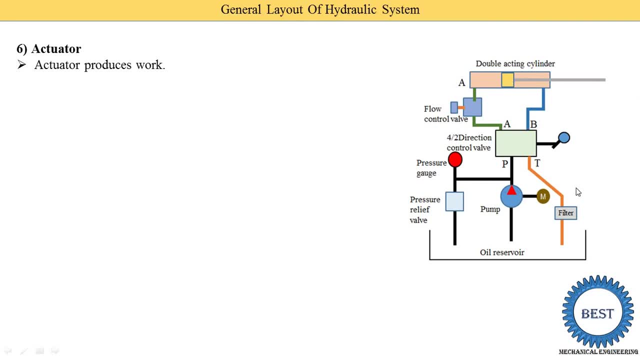 here get this mechanical energy, okay. and in a pump we supply mechanical energy and here get we mechanical energy. so some person is think that directly we supply this mechanical energy here, okay. why we are required is much of the systems. so for that you comment on this video. what is your? 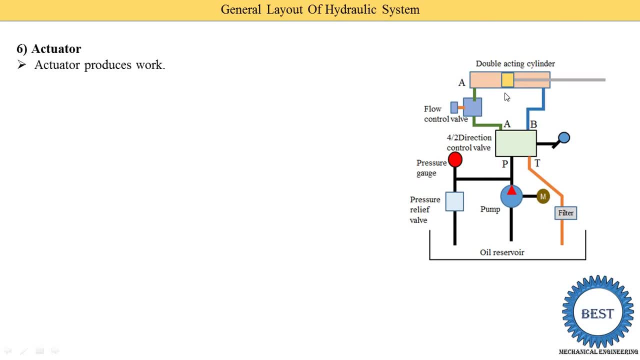 answer why we supply mechanical energy as a input to the pump and we also get the mechanical energy. there are a two types of the accutators. one is the linear accutators and the second is the rotary accutators. linear accutator is called as the cylinder. okay, so here you read this word: that 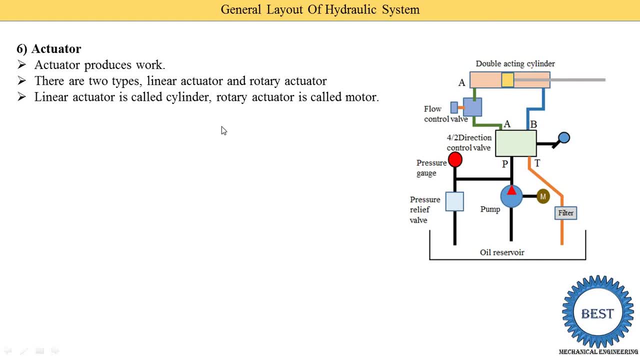 is double acting cylinder. so this is our linear accutators, and the rotary accutator is called as the motor. okay, so in a next few chapters we- you hear this word accutators. what are the various types of accutators? so hydraulic motor is also there. okay, you only need here, you only need to. 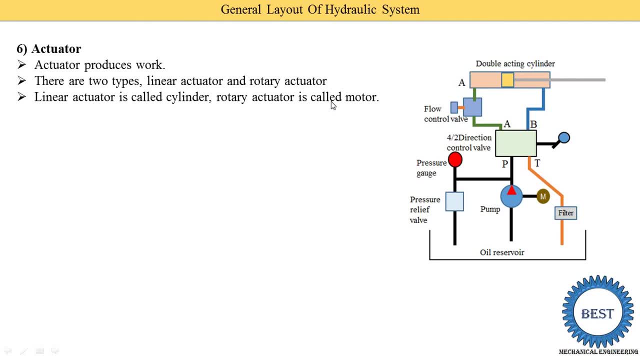 the name is. that is electric motor, is there? okay, but hydraulic motor word is also coming in a few chapters, okay. so what is the meaning of hydraulic motors? it is the rotary accutators. okay, so rotary accutators is also called as the hydraulic motor. double acting cylinders develop the force and 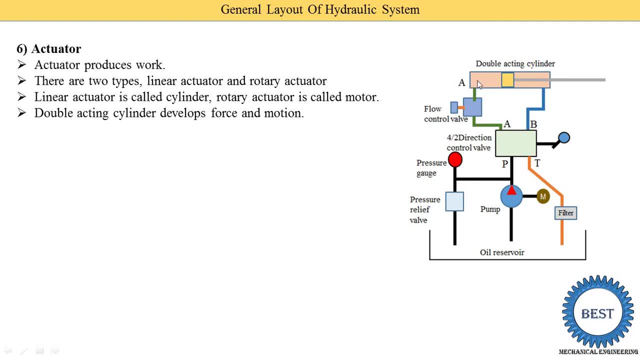 motions. okay, so here we supply some quantity of the oil and it's converted into these mechanical motions. okay, so this piston is reciprocated. with this piston, this connecting rod is also reciprocated and here some force is created. so how amount of the force is convert? 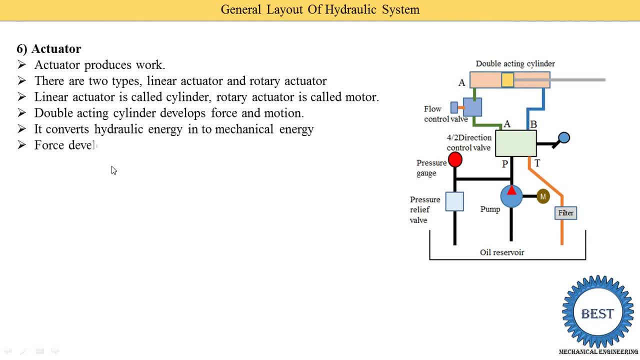 so it have the equations. which equation? force developed is equal to pressure of oil, and is sorry, force developed is equal to pressure of oil into area of the pistons. okay, so here we see that the force developed is directly proportional to the pressure and the area. okay, so if we increase, 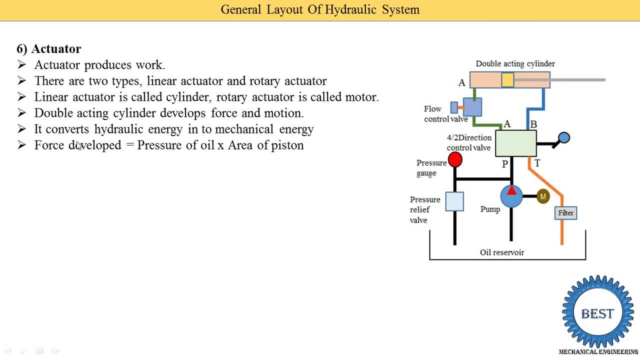 the area, force is increased. if we increase the pressure of oil, the force is increased. okay, so are going to increasing and increasing the pressure of the oil we are able to achieve the more force. okay, suppose we require more force. we have only one option: to increase the pressure of. 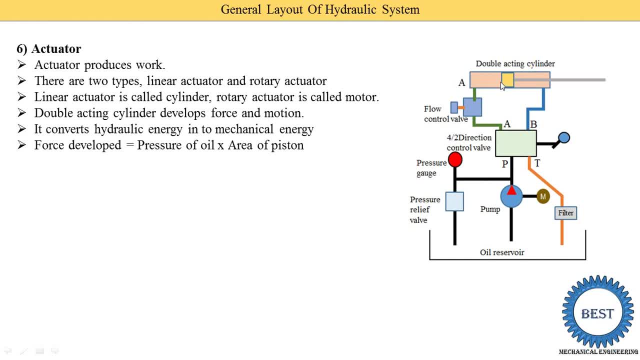 the oil because the area of the piston is fixed. we are not going to change the area of the piston. okay, because it is a fixed component, is there. so we have only one option is that if we want the more force, we increase the pressure of the oil that supplied to the accutators. okay, and in? 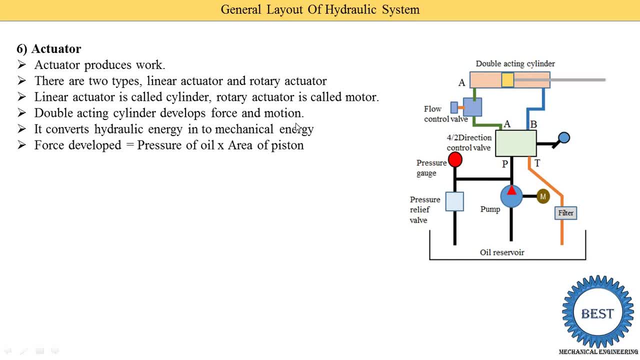 accutators the hydraulic energy into the mechanical energy. okay, means we supply hydraulic energy into accutators and it is converted into the mechanical energy. next component is the pressure gauge. so you already know what is the function of pressure gauge. it is an important components of hydraulic system. it show the pressure reading. okay, why it is important. 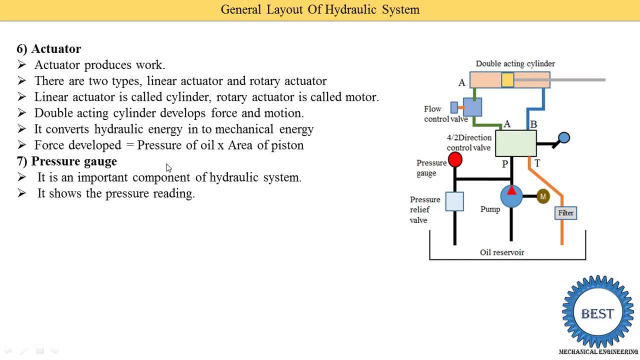 we are not only written. it is important. okay, it have some reasons that why we written. it is a important components because without measuring the pressure the pressure relief valve is not operate okay and if the pressure is increased, then the desires. then are also chances of the collapsing of the systems or damage or leakage. 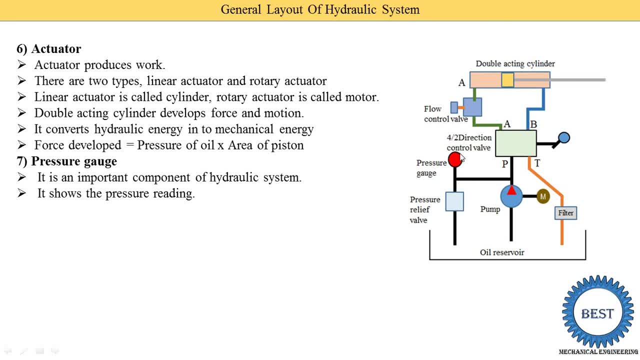 is created inside the system. so it is most important thing is to maintain the pressure inside the any hydraulic systems. so pressure settings are made by locking to the pressure gauge. without pressure gauge it is not possible to make the pressure relief valve setting and unloading the valve settings okay. so without 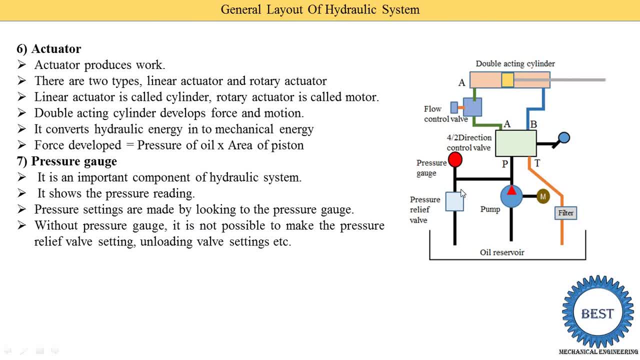 pressure gauge, the pressure relief valve is not operate. okay, because they are. pressure relief is required to sensing of the pressure and this sensing is done by using the pressure gauge. that's why this pressure gauge is most important. and the last component is the filter. main function is to remove suspended solid contaminates from the oil and it and to provide 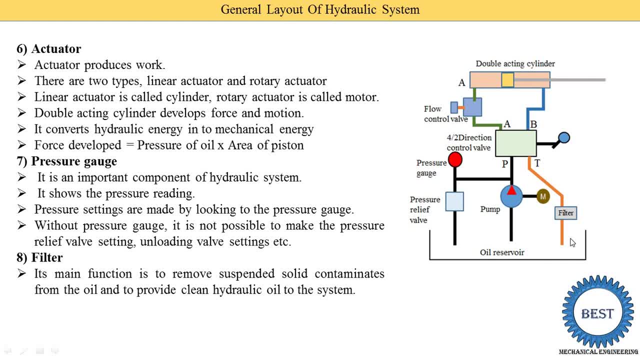 clean hydraulic oil to the systems means the filter is generally used to remove the suspended solid contaminates from the oil and supplied the clean oil to the systems. so in a some book the filter is provided in this return pipe and some book it is a putted in a supply pipe of the pump. okay, so both the locations are correct. you not need. 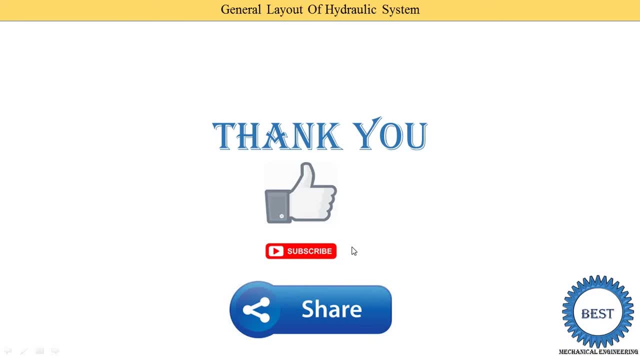 to the confuse about it. so thank you for watching this video. if you learned and like the video, subscribe the channels, comment on the video and don't forget to share with your friends.